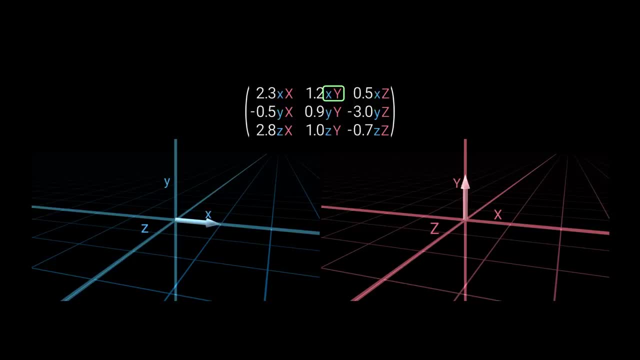 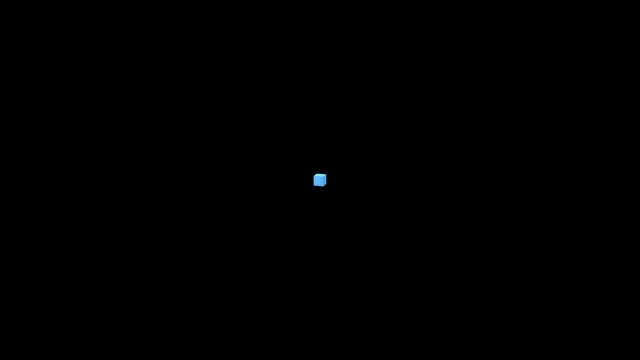 them. We'll gradually clarify this relationship as we continue. Similarly, this one is associated with the z-axis of the blue space and the x-axis of the red space, And we have here all nine possible combinations. Now let's put it to use with an example. 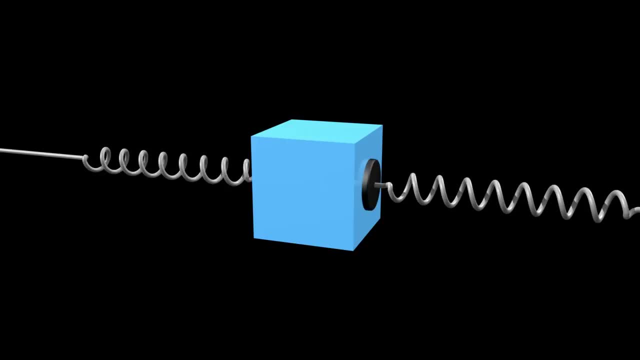 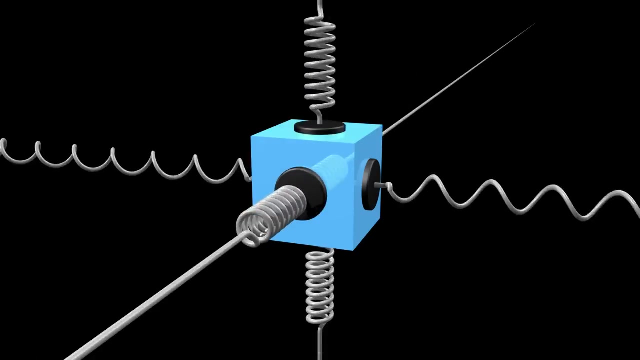 Here's a tiny metal cube. Let's attach strings to it And pull. This stretches our cube a tiny bit, though the effect is too small to be shown here. Now we're compressing it. We can independently stretch or compress the other faces. 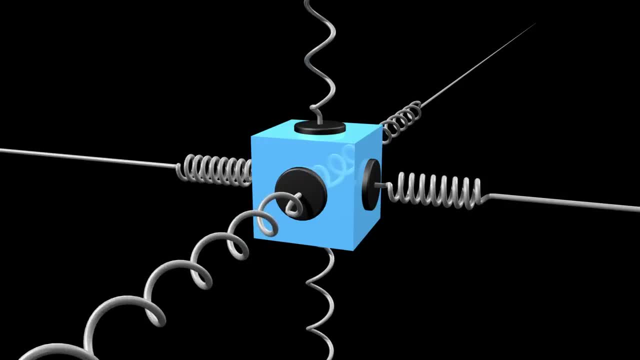 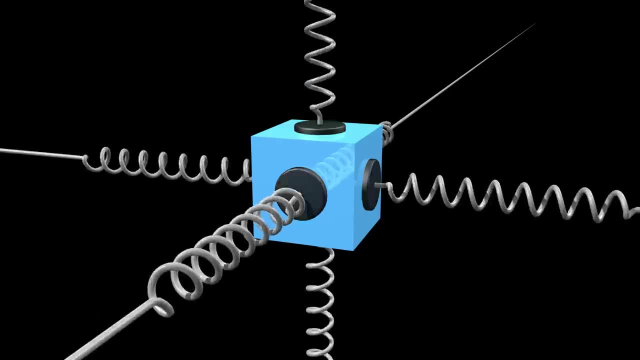 But we always make sure to keep the cube in equilibrium so it won't move. If we apply a force on one face, the opposite face gets the opposite force. We can also pull this way. This generates what's called a shearing force. 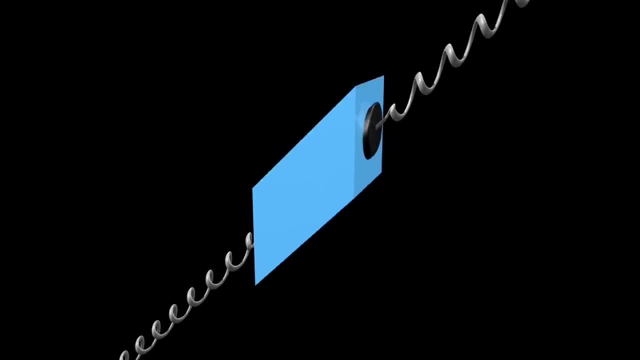 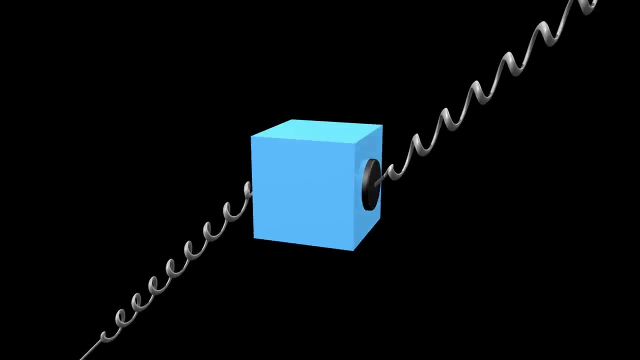 This generates what's called a shearing force. Such a force attempts to deform the cube like this. Of course, in reality, the cube will simply rotate. But we want our cube to be in equilibrium. It shouldn't move and it shouldn't rotate. 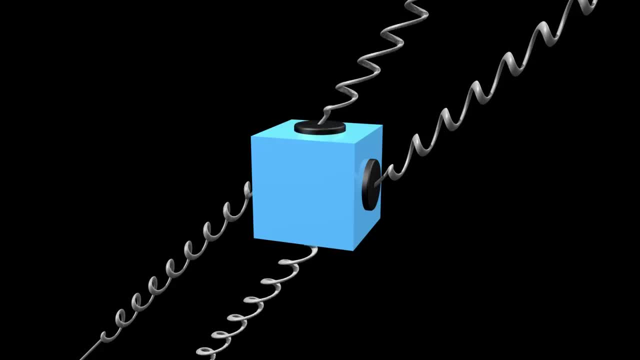 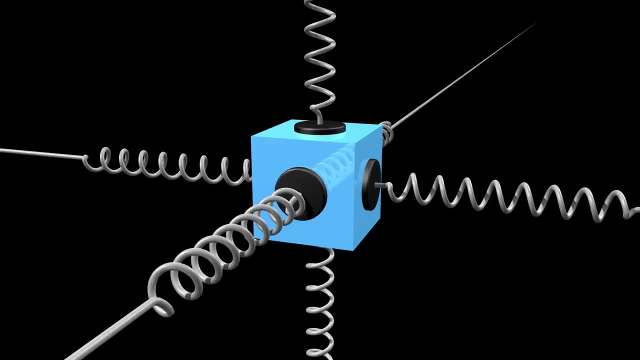 So if we want to apply such a force, we'll need to balance it with another shearing force acting on the top face. The forces acting on the cube faces are called stress forces. There are many ways to combine them while keeping the cube in equilibrium. 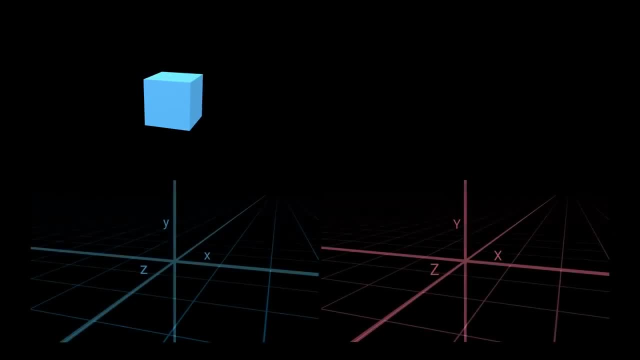 Now let's model this using what's called a shear force. So let's look at the shear force. We'll use 2 vector spaces. again, We can think of the blue one as responsible for selecting a face. The red one will specify a force. 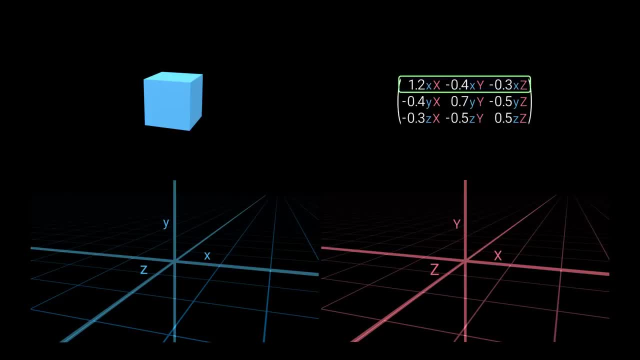 And here's an example: stress tensor. The first row is entirely labeled with blue X's. This means it is associated with the face pointing in the X direction And it contains the 3 components of force. This is the force acting on the cube. 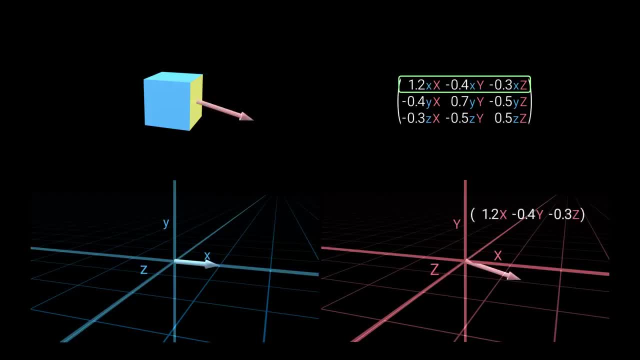 Now, if we were to take the cube and put it on this piece, then we'd have the whole force of force in equation 4.. acting on this face. The second row is entirely labeled with blue Ys, so it similarly defines the force acting on the top face. 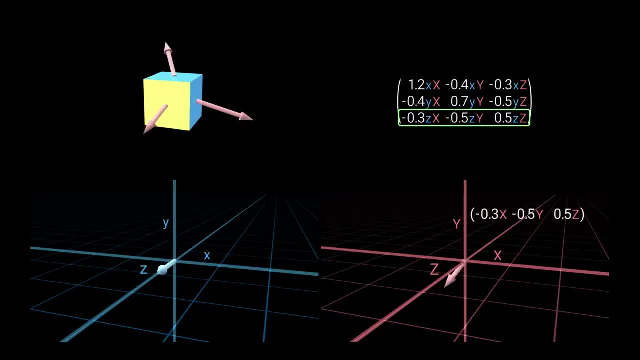 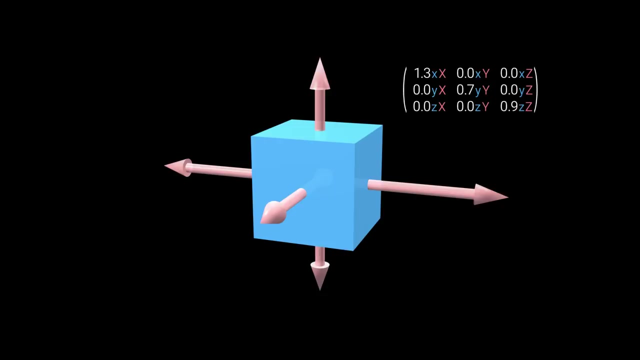 and the last one on the front face. We assume the forces are balanced to prevent motion, so the opposite faces get the opposite forces. Stretch and compression forces are specified by the diagonal of the matrix. That's because the direction of the face and the direction of the force are the same. 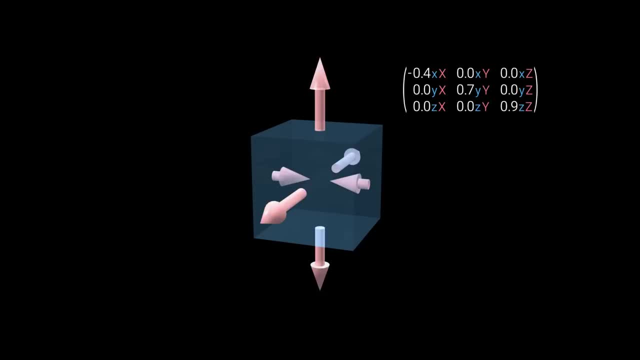 A negative value indicates a compression force and the arrows face inward. Shearing forces are specified by matrix elements that are off-diagonal. Here's a pure one. Recall that we need to balance them to prevent rotation. This makes the matrix symmetric around the diagonal. 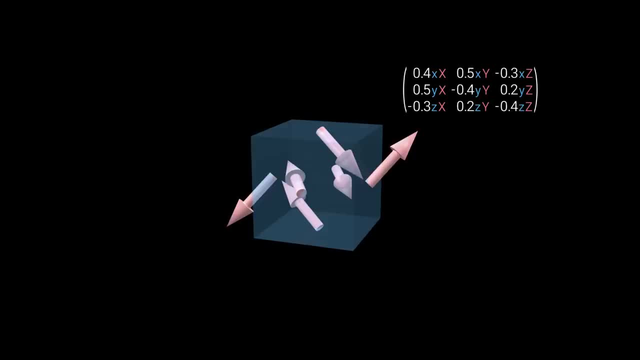 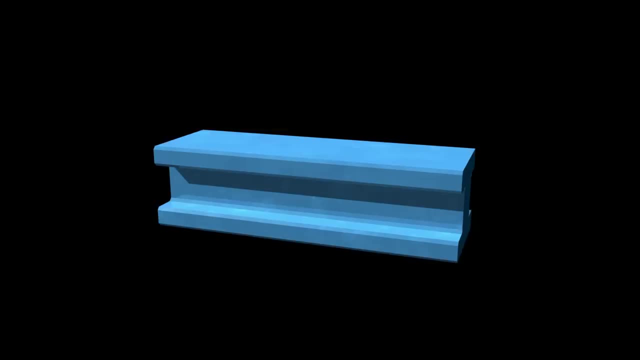 Any symmetric matrix represents a valid stress tensor. This cube is not really an ordinary object. It's actually a small region inside an object, such as a beam of a bridge. This beam is under stress due to the load it carries. Our tensor describes the stress forces felt. 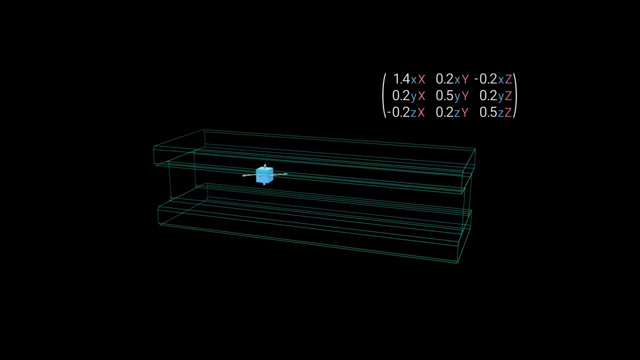 at a particular small region inside it. Different regions may experience different stress forces, so each one has its own stress tensor. The regions are actually infinitely small, so each stress tensor describes one point in space. Now let's focus on the original point we started with. 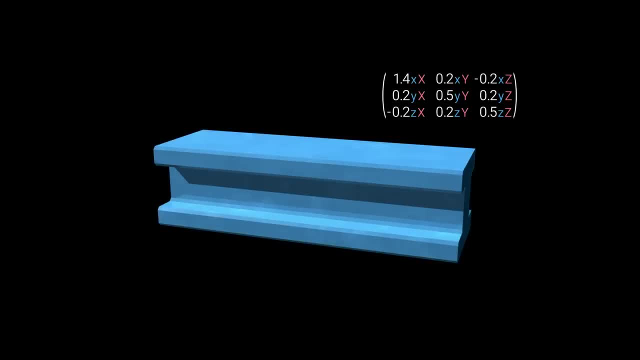 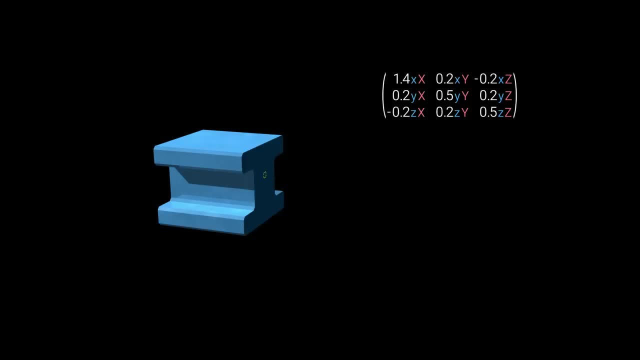 Of course it's hidden inside the beam and we can't directly observe it. but imagine we could slice the beam open and peek at the stress forces inside. Let's mark the point our tensor describes, Since we revealed the face pointing in the X direction. 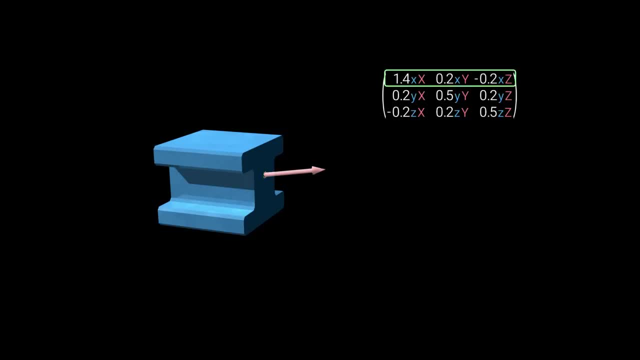 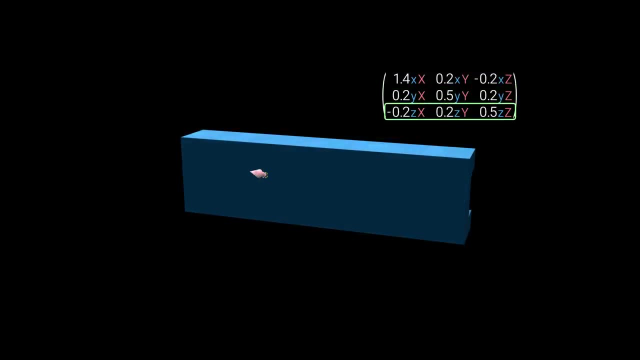 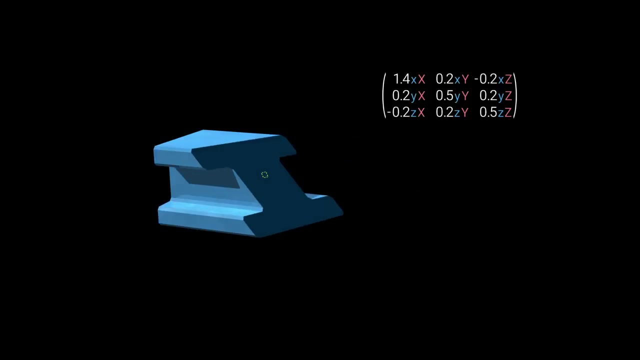 we'll see the stress force specified by the first row of the matrix. And now we see the force specified by the second row and now the third. But what if we slice diagonally? This slice is not aligned with our axes, but our choice of axes is arbitrary. 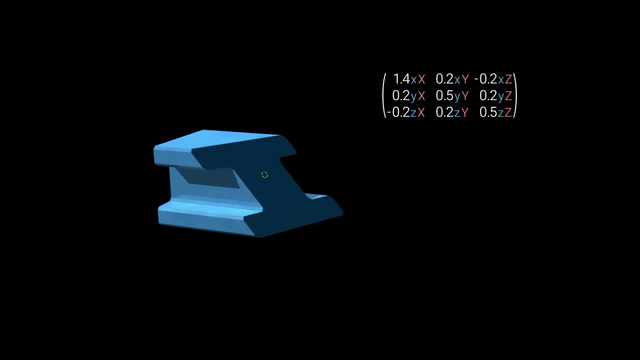 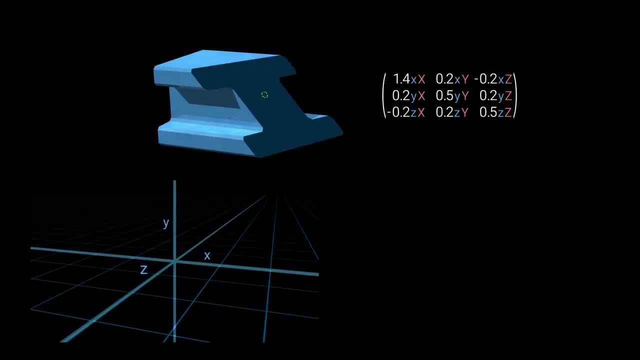 So this slice is as good as any, and we should get some stress force here too. Our tensor gives us this information as well, according to the following rule: We exposed a face pointing in the direction of this vector. Its components are 0.7,, 0.6, and 0.4.. 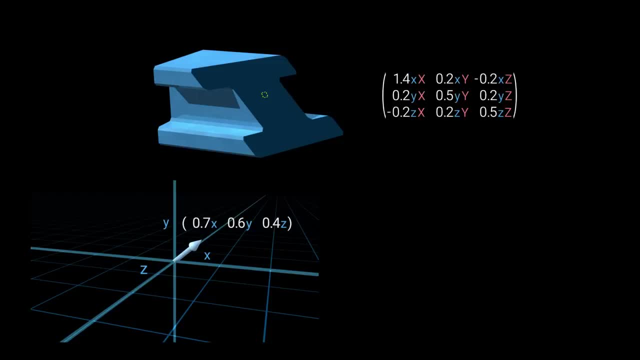 The stress force acting on this slice is the weighted sum of the three forces specified by our matrix. So we need to take the first row, scale it by 0.7, which means multiply by 0.7.. Multiplying each component by this value. 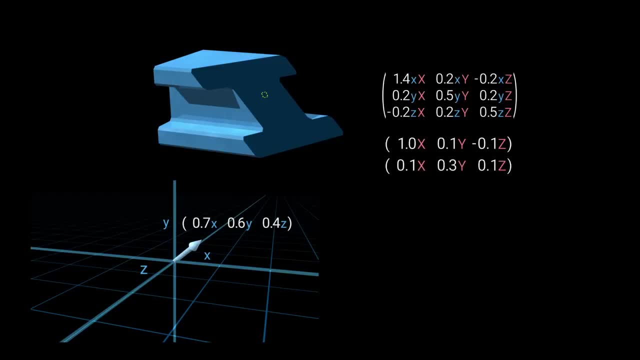 Scale the second row by 0.6 and the third by 0.4.. Then add them together And this is the force acting on our slice. This computation is the same as vector matrix multiplication. So now let's try a new visualization. 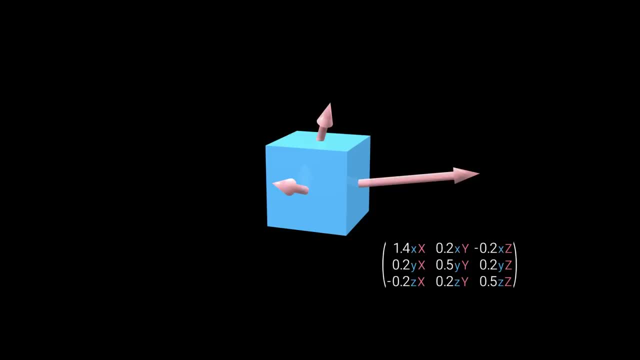 Previously we've drawn the three stress forces specified by the rows of our matrix on the faces of a cube. Now let's draw the same forces on a sphere. We can compute forces in other directions using the rule we just saw as a weighted sum of these three. 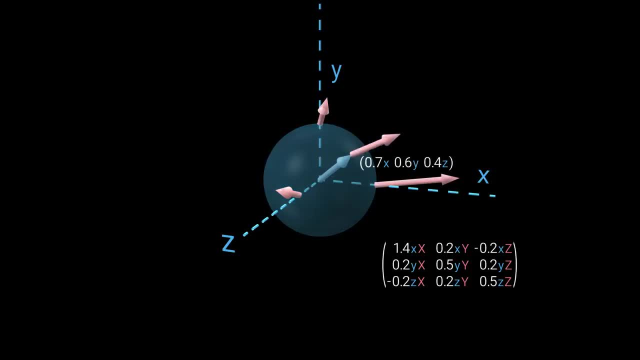 Here is, for example, the direction we just saw and this is the force we computed it to be. And here's another example: Since it's closer to the y-axis, the y component is large and the stress force here will be more similar. 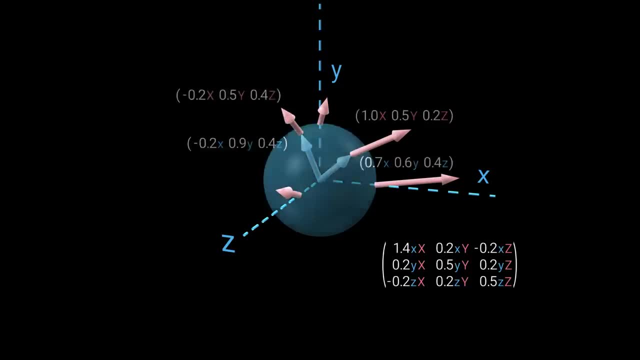 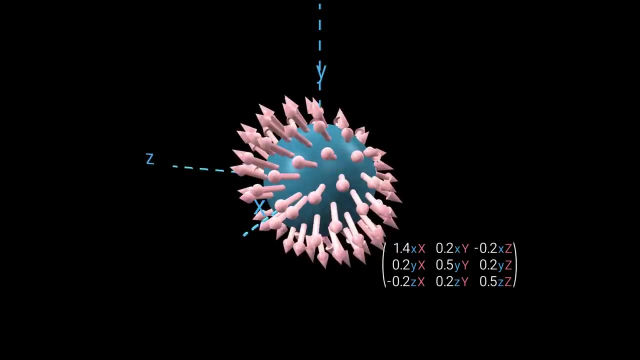 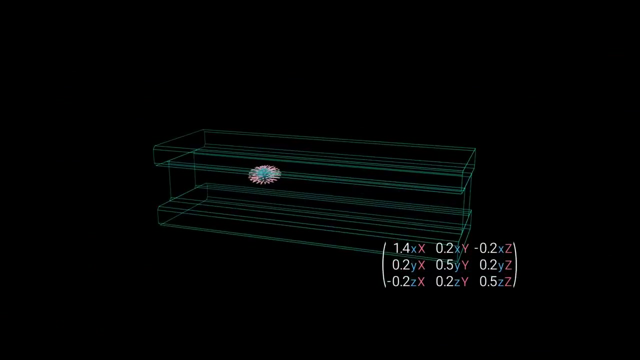 to the force at the top. So let's draw them all around the sphere. This is a good visual metaphor for what a stress tensor really is. It shows the stress force felt in every possible direction. we can slice the beam. We'll soon show what it looks like. 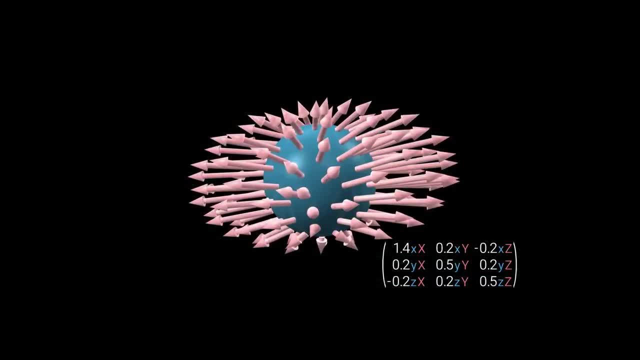 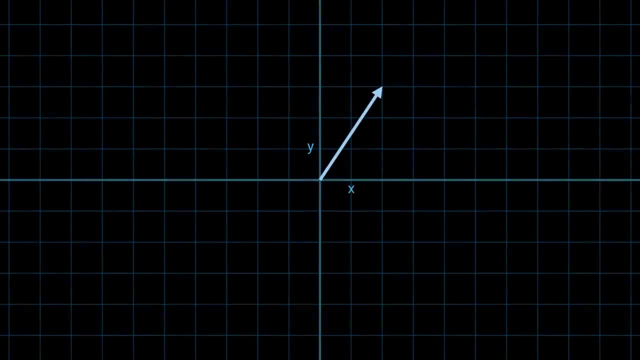 for various values of the matrix. but first here are some general notes about tensors. Let's return to vectors for a second. We said we can visualize them as arrows or specify them using an array of components, But these components are not all the same. 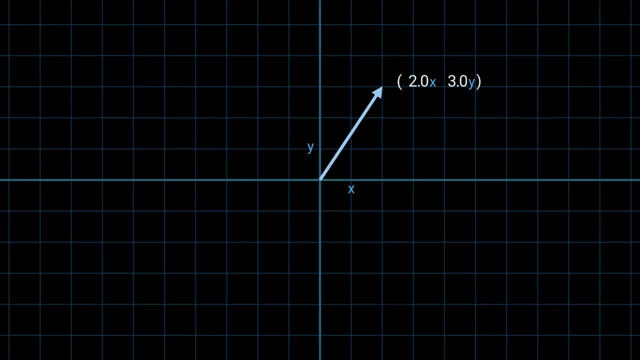 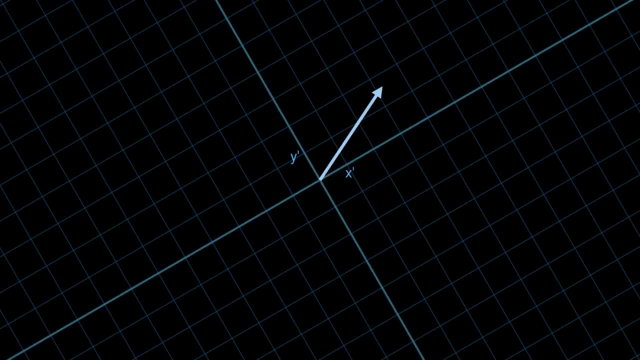 They're not all the same, But these components depend on our arbitrary choice of axes. We can choose different ones. Here's, for example, a different coordinate system. We'll call the axes here x prime and y prime. Here the vector has different components. 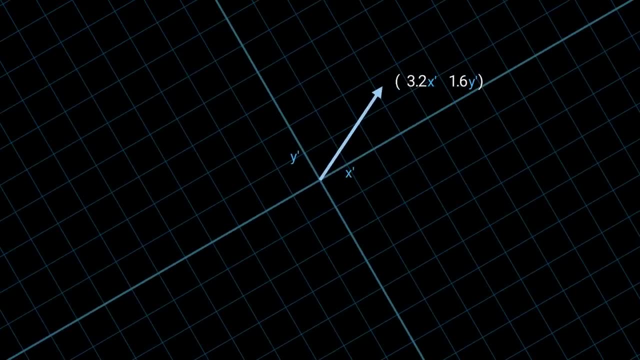 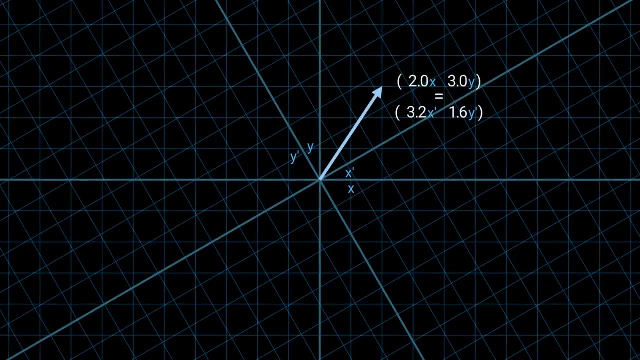 But note, our vector didn't change. We just changed the coordinate system and rotated the camera So we can write this equality. These are two different ways to represent the same vector. The same thing is true for tensors. We have a visual representation of a tensor. 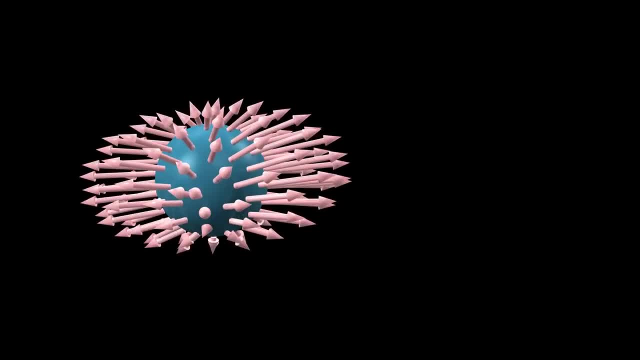 We can change our point of view, but this doesn't change the object, And we can also represent a tensor using an array of components. This representation does depend on a particular coordinate system. The array describes only three vectors, those that happen to lie on our chosen axes. 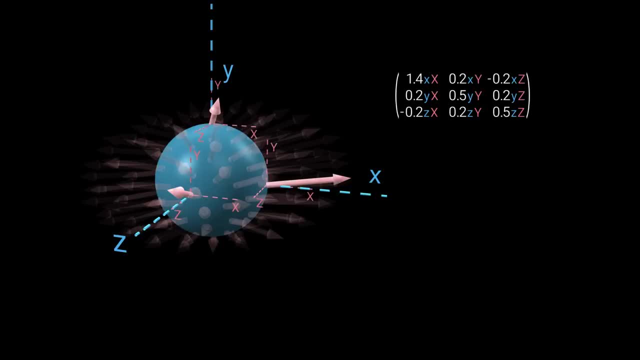 And they're broken down into their components using the same coordinate system, ending up with nine components. The rest of the vectors can be deduced, but not all of them. The rest of the vectors can be deduced, but not all of them. 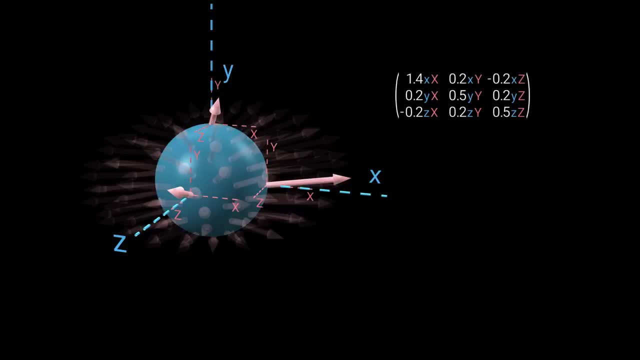 The rest of the vectors can be deduced- but not all of them- using the weighted sum rule. So this array describes the tensor in full. We can choose a different coordinate system And we'll get different components. We can say this system describes the tensor. 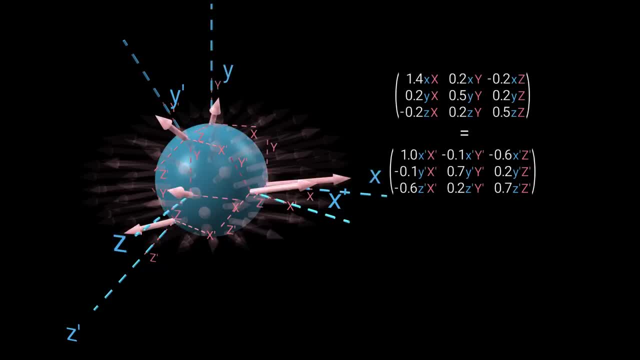 from this point of view, And we can write equality here too, It's the same tensor. There are formulas for transforming an array, given how our coordinate system has changed. This is especially useful in relativity, where switching between two vectors, between coordinate systems, is crucial. 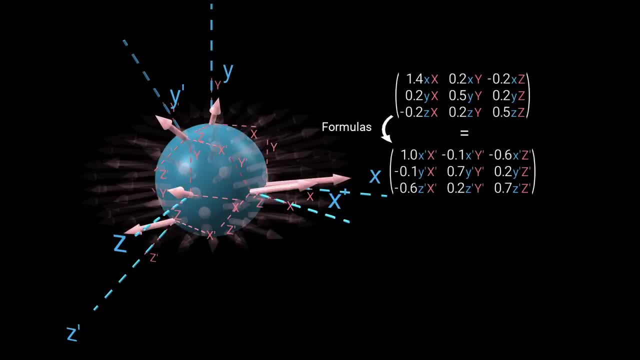 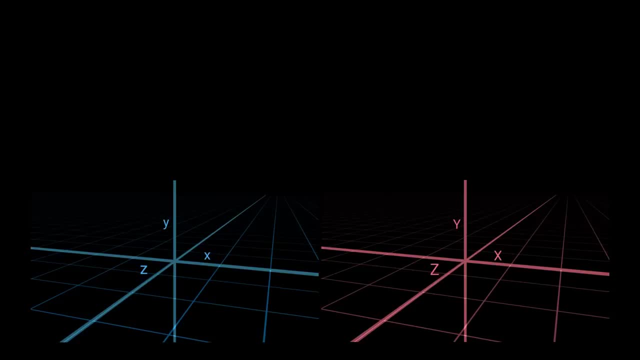 In this video we've only shown simple rotations. Later we'll show scaling and skewing as well, where things get more complicated. Also, we only constructed tensors over two vector spaces. These are second-order tensors. Here is a third-order tensor. 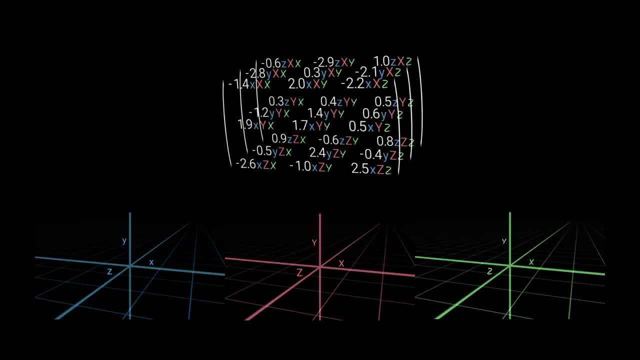 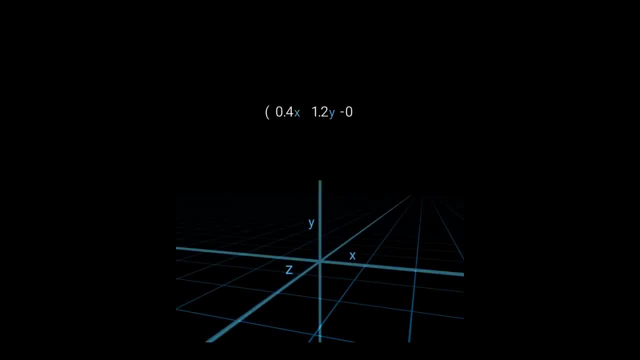 It has 27 components, one for each combination of labels from the three spaces. We are yet to explain the full meaning of these label combinations. A first-order tensor is simply a vector And, of course, everything works with spaces of any number of dimensions, not just 3D. 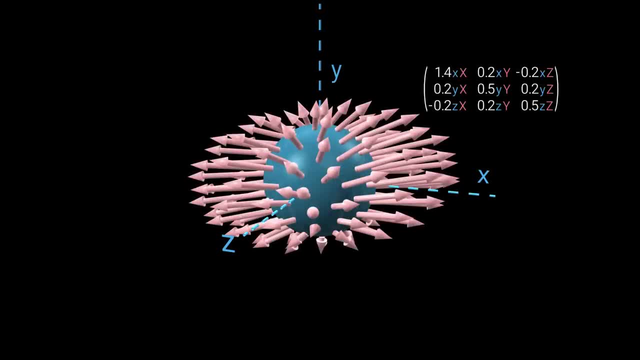 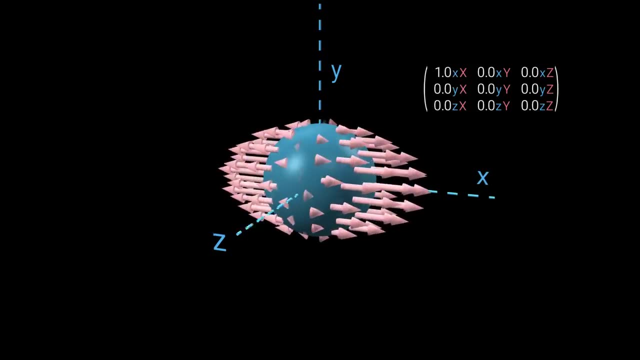 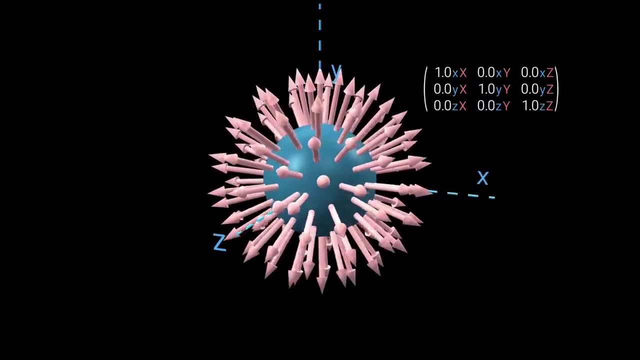 Now let's visualize second-order tensors. Let's think of it as a stress tensor. for now We'll start from an all-zero matrix and add components of the diagonal one by one. Each component of the diagonal controls the space. Each component of the diagonal controls the space. 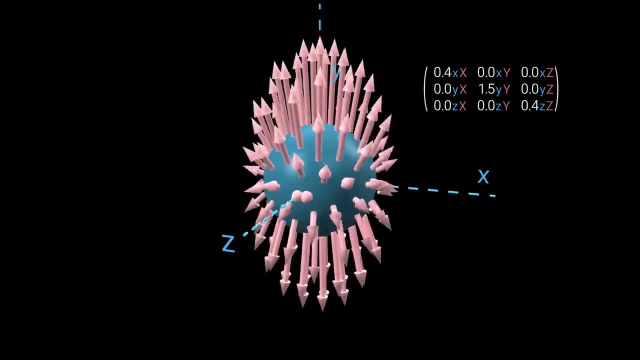 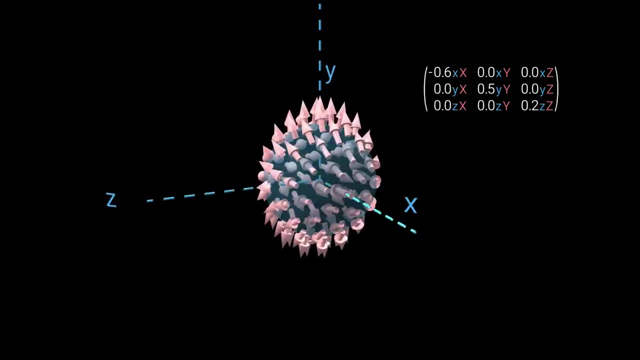 We can define the size of the bulge along one axis. We can define the size of the bulge along one axis. We can define the size of the bulge along one axis, And we can also have negative bulges, And we can also have negative bulges. 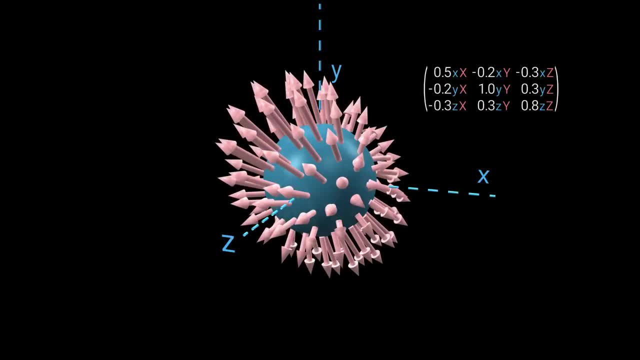 Now let's add shearing forces off diagonal components, but we'll keep the matrix symmetric as required for a stress tensor. The forces that lie on the axes are slanted now because they contain shearing components, But overall we got the same kind of oval shape.